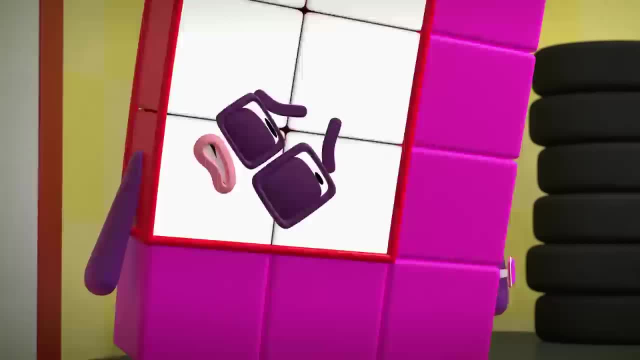 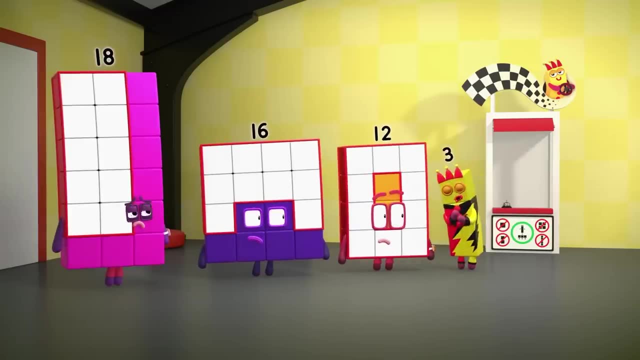 Oh, can you please move faster. Some of us can't wait to go go-kart. Hey, hey, hey, I'm going as fast as I can. you know, Subtracting threes one by one is a slow business, I mean. 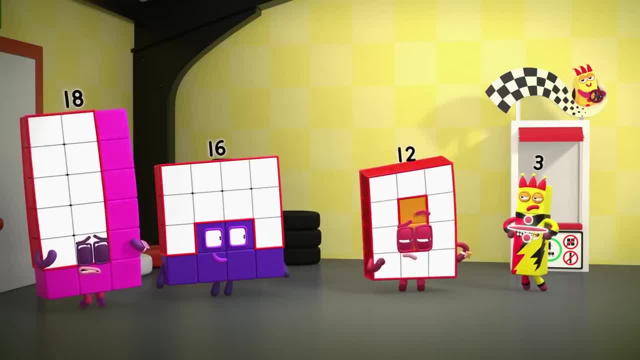 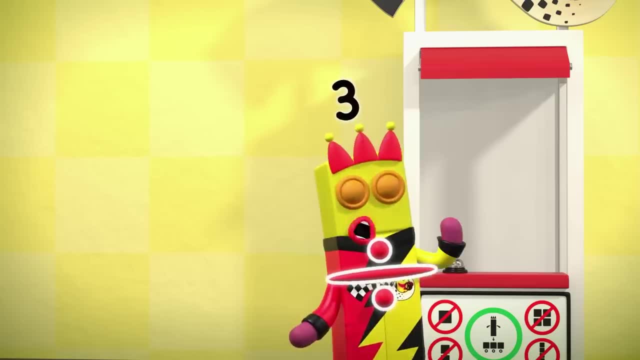 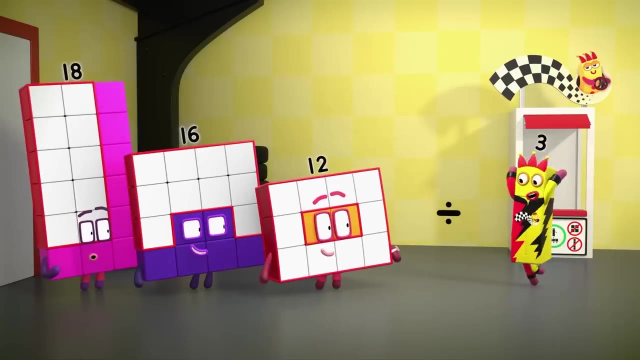 if you know a faster way of dividing into threes. you tell me Time. Oh, I know Juggling helps me think. Oh, it's a sign, A new sign. Maybe this can help me divide into threes. Let's see, Look, can't you see? I'm keen to try something new Instead of taking threes. 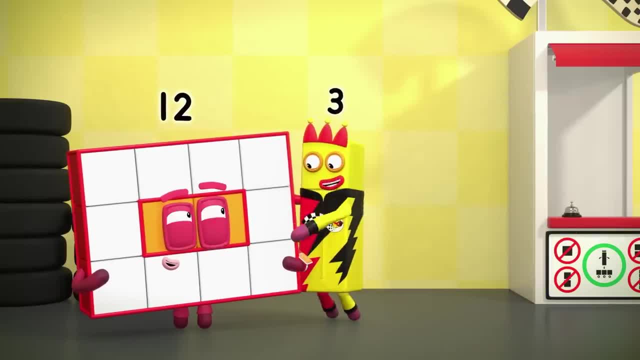 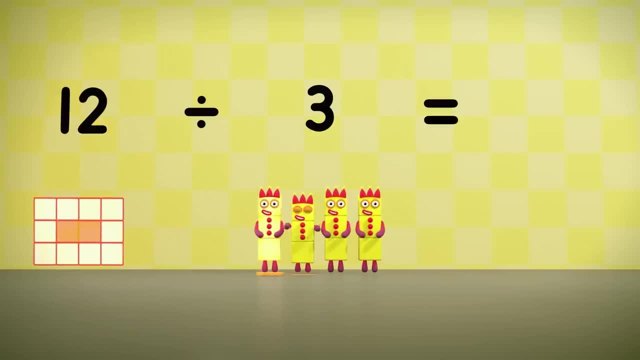 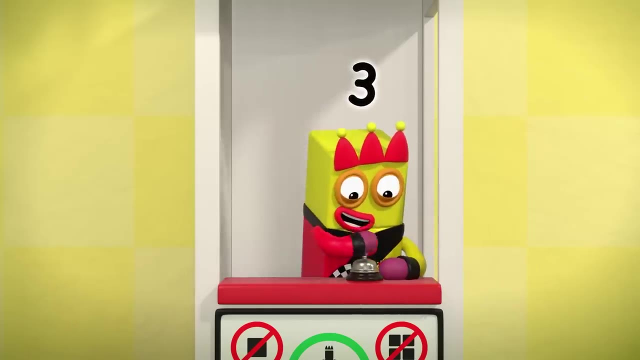 away over and over. let's divide you into threes all at once. Twelve divided into threes equals one, two, three, four. There are four threes in twelve. Woo-hoo, Woo-hoo, Woo-hoo, Woo-hoo. 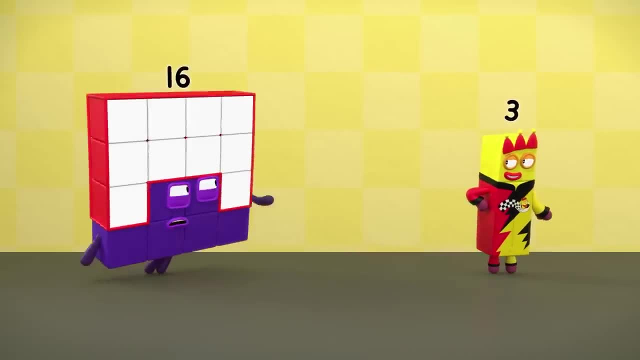 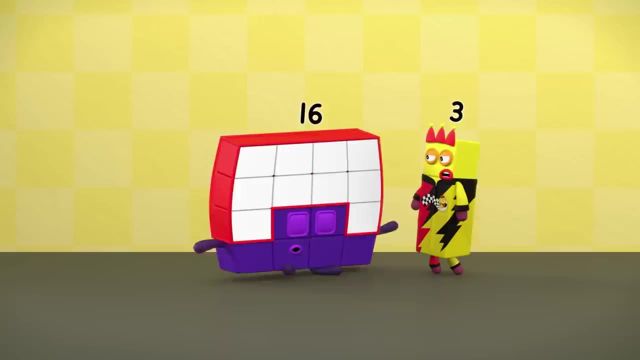 Woo-hoo, Woo-hoo. I can divide anyone like this, Anyone. you say Why I'm anyone? Give it a go. Sixteen, No, no, no. You need to make a rectangle that's three blocks high, like twelve did. 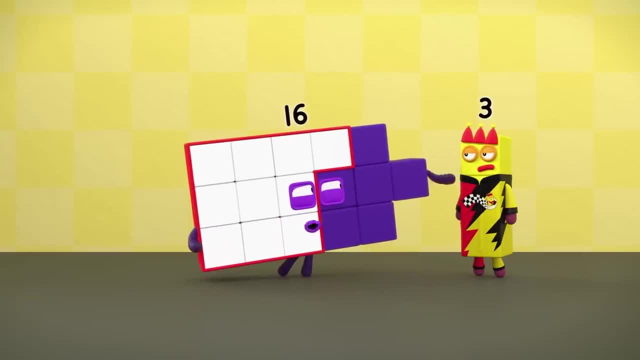 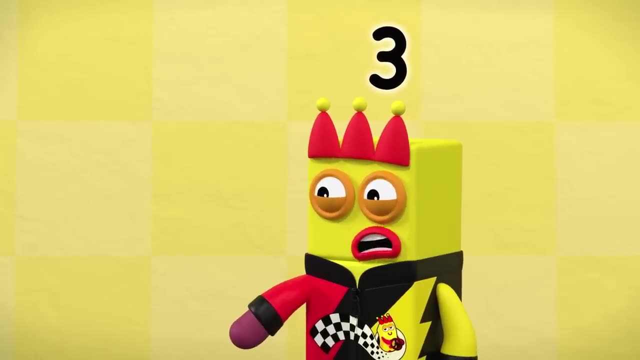 Nope, Not going to happen. Got this one block remaining on the end. I guess I can't divide you into threes without leaving some of your blocks behind. Sorry, sixteen, but you won't be able to divide me into threes. 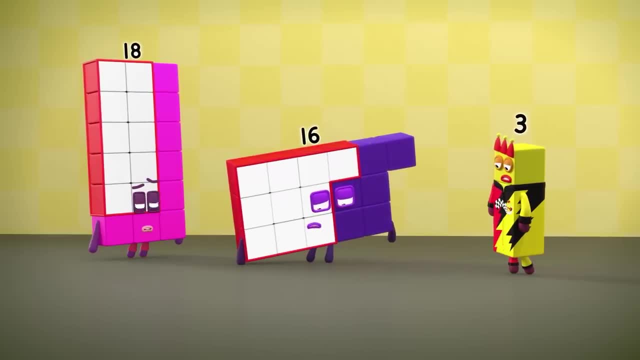 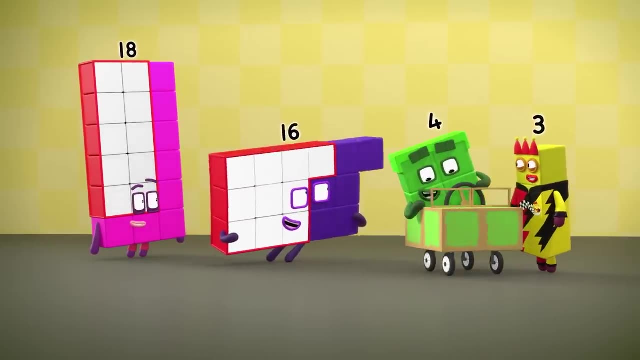 You won't fit in my go-karts, Oh, excuse me. Coming through, Who wants to go on my go-kart track For four-wheel drivers? Oh, can I try? Sorry, three, Only fours can drive my karts. 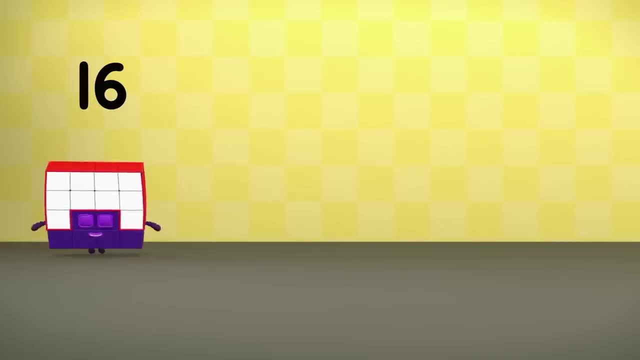 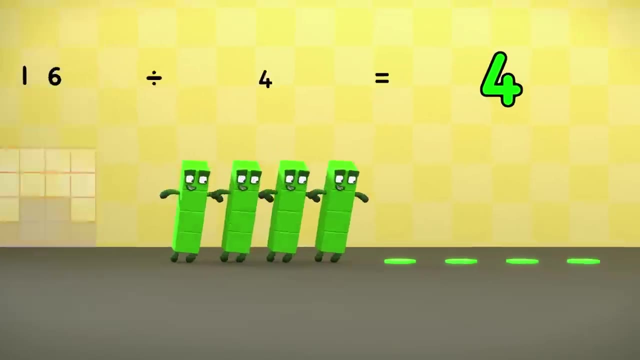 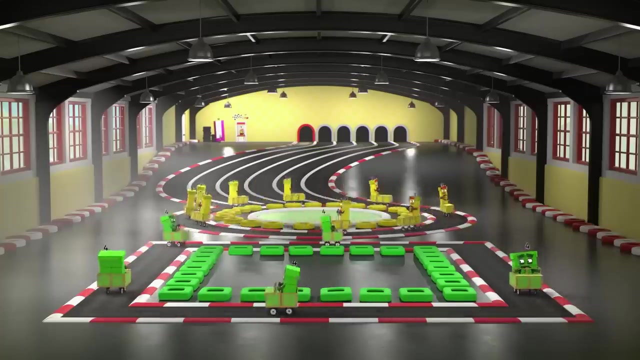 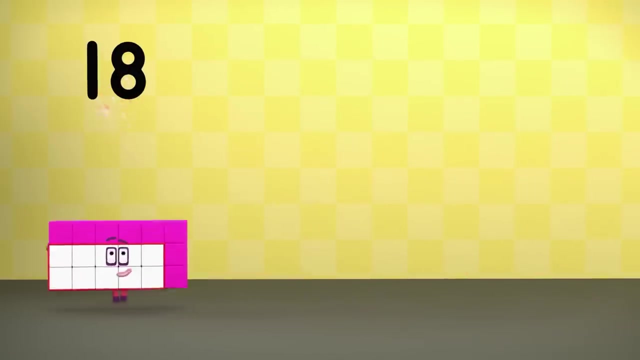 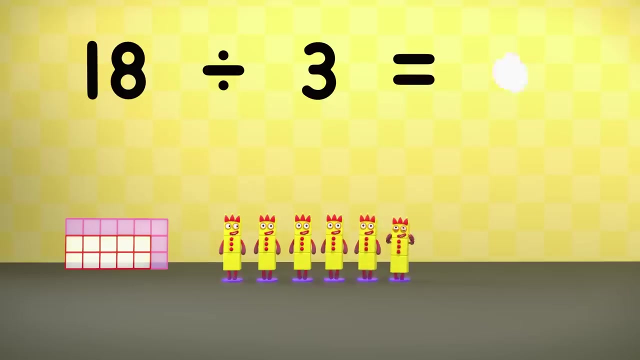 Oh, maybe I can. Sixteen divided into fours equals one, two, three, four, The four fours, The four fours. Oh yeah, Woo-hoo, Literally unable to wait a moment longer. Eighteen Divided into threes equals one, two, three, four, five, six. 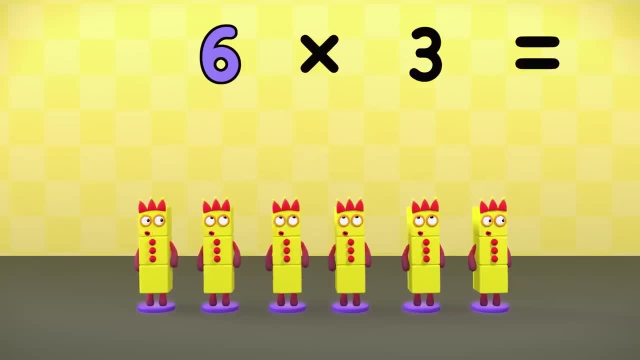 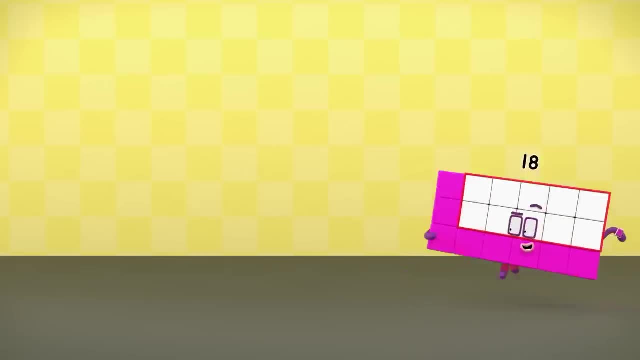 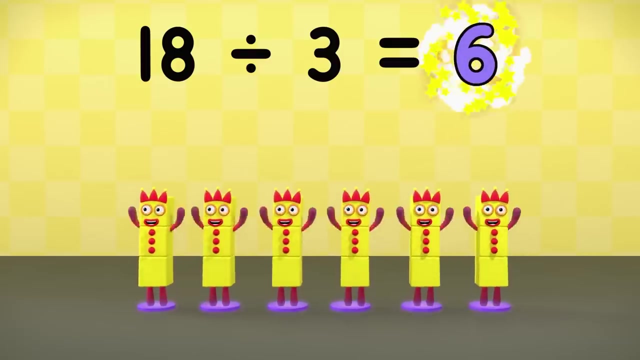 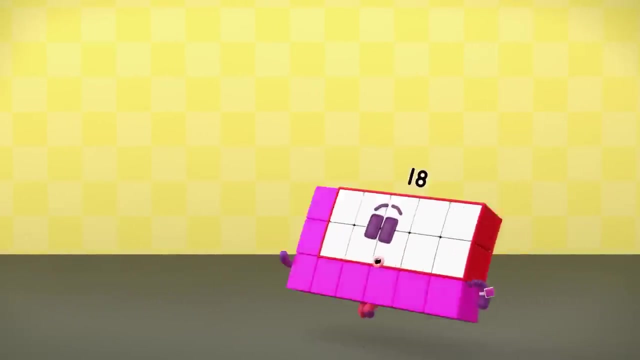 All right, yeah, Six times three equals Eighteen. Eighteen, What do you know? Division is the opposite of multiplication. Here I go again: Eighteen Divided into threes equals six. Six times three equals Eighteen. I could do this all day, so I will Eighteen. 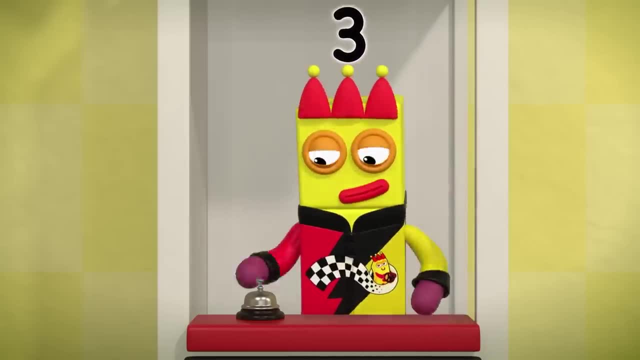 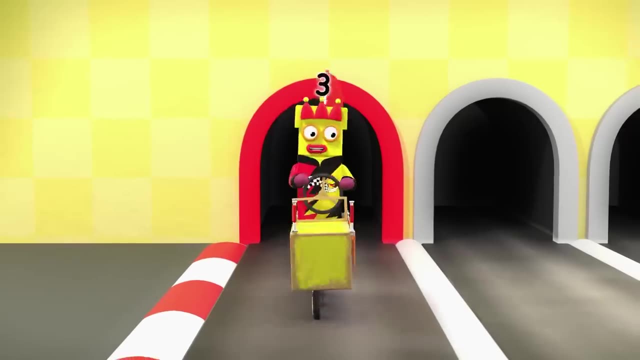 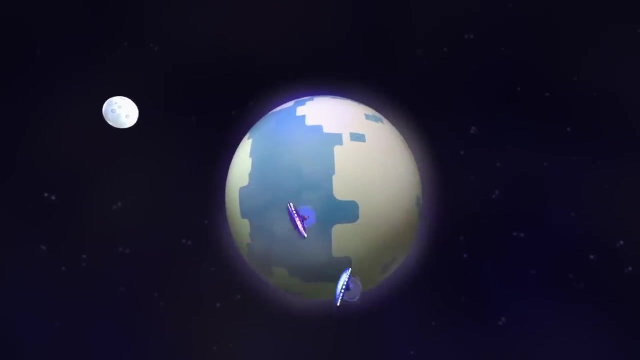 Divided into threes equals six. Some rulers are just born to show off. Six times three equals Eighteen. Eighteen Divided into threes equals. Divided into threes equals. Look at me, How many twos is too many twos, amigo. 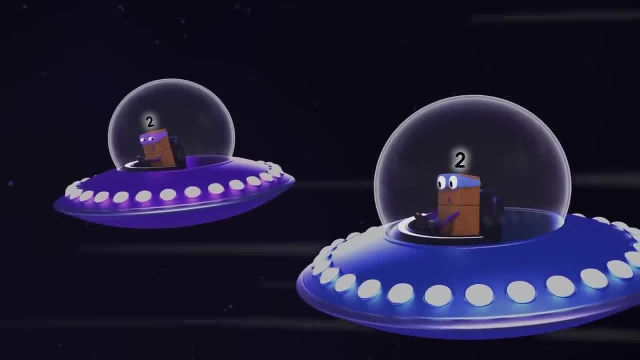 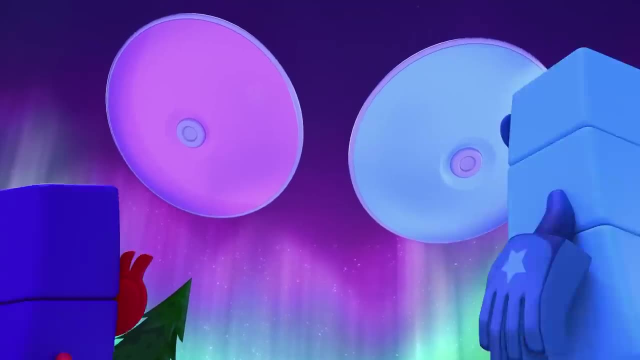 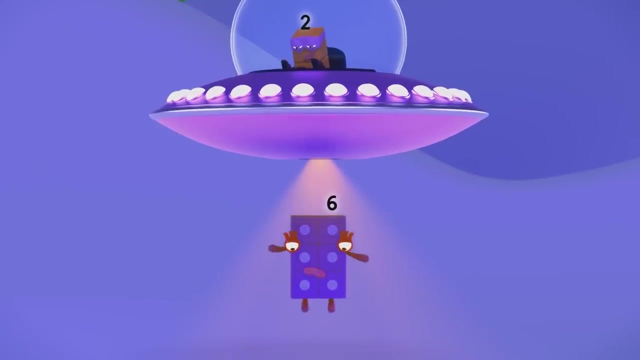 Let's find out with a game of how many twos- One, two, three, four, five… Huh, Oh, my ded allemaal. You said that anyway, That that I kept saying…. Let's find out how many twos there are in six. 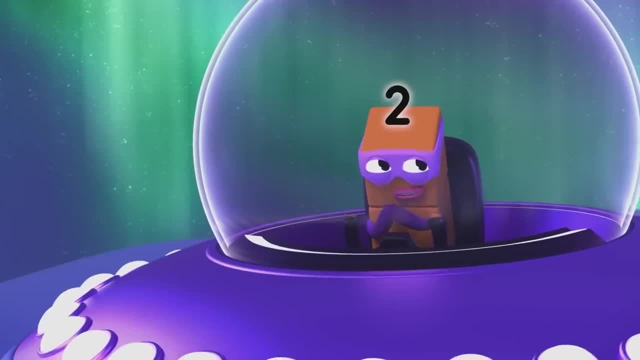 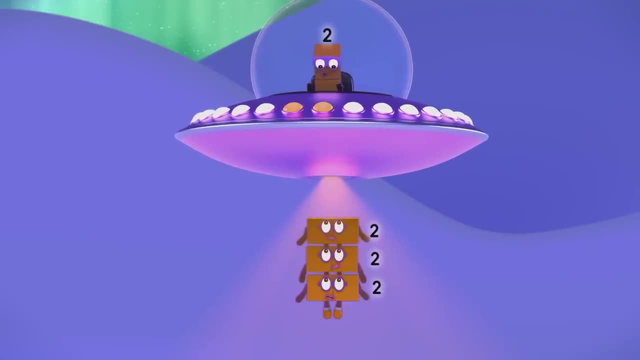 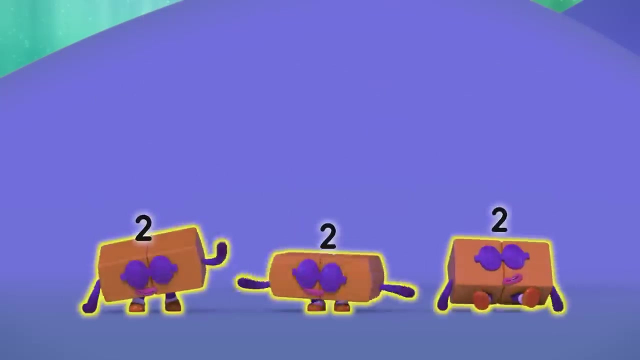 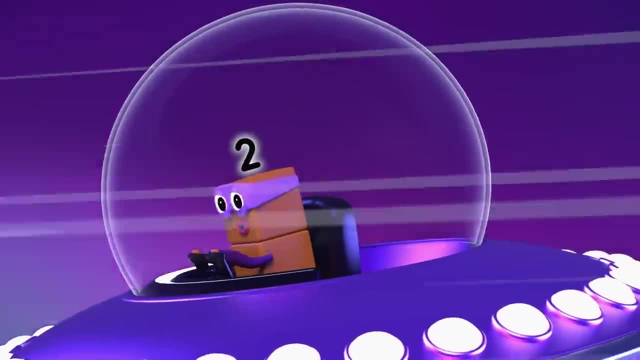 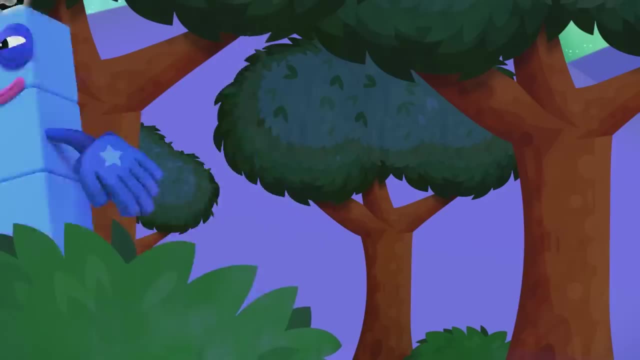 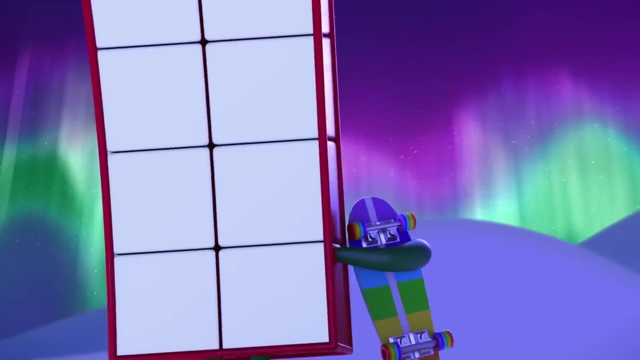 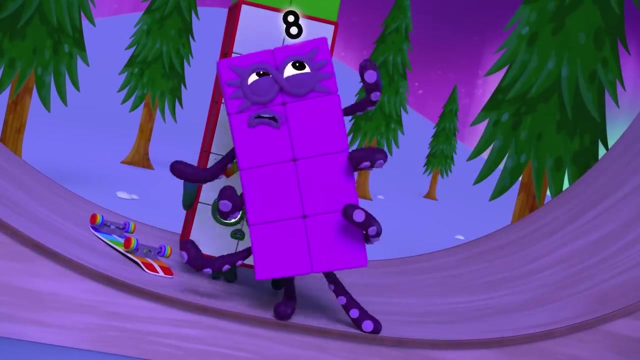 Happy Terrible Tuesday everyone. Happy Terrible Tuesday everyone. Of course, should that be every two Woo-hoo, Hey-hey, Whoa. Target acquired, Oh, Never fear, Fourteen. I've dealt with the Terrible Twos before. 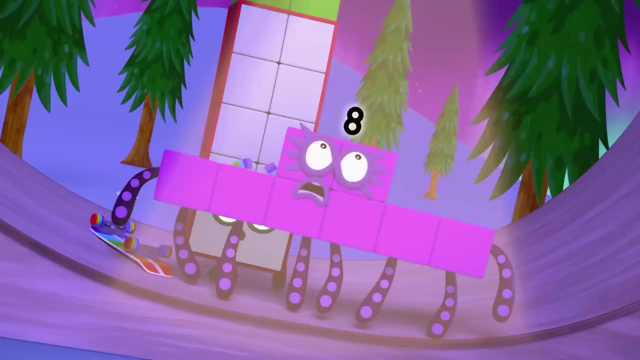 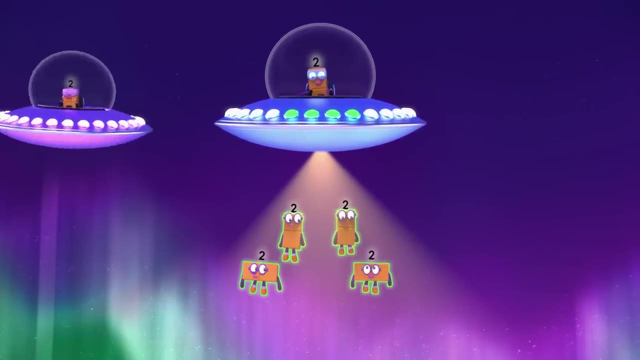 Off to block shield. One, two, three, four, five, six, seven, eight, seven, eight. One, Okay, two, three, four, Hey, Hey. Hey, There are four twos in eight. You're in the lead, amigo, but not for long. 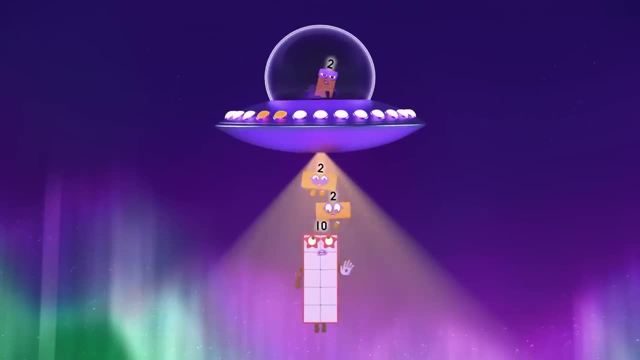 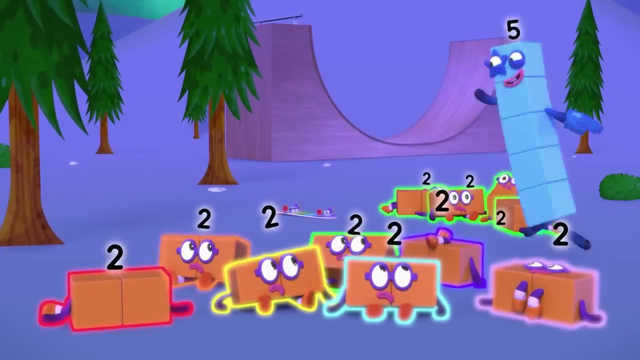 Woo-hoo. One, two, three, four, five, six, seven. Oh pretty, There are seven twos in 14.. Beat that, Whoa. Whoa. Excuse me, I need to lend a hand. 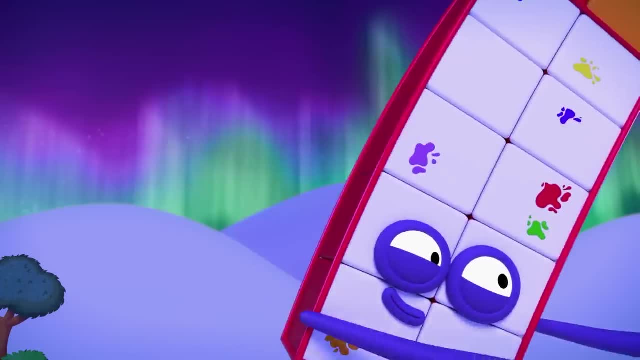 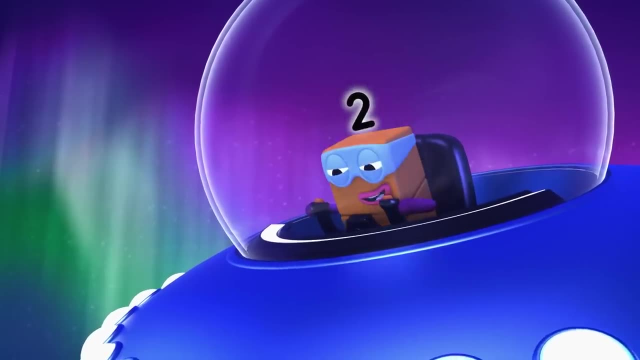 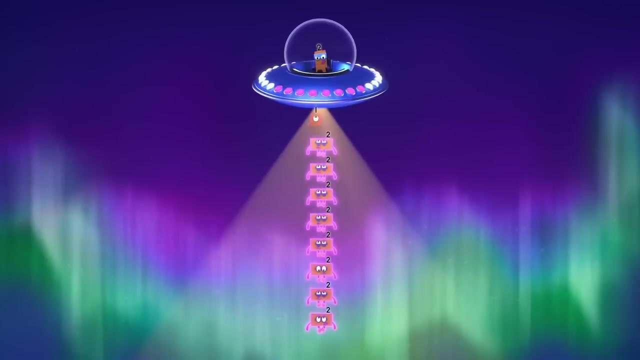 Ooh, Whoa, Ooh. Hold, still, 17 is greater than 14.. So this should put me back in the lead. Hey, Ooh, Hey, Remainder alert, Remainder alert. There are eight, twos in 17 and one left over. 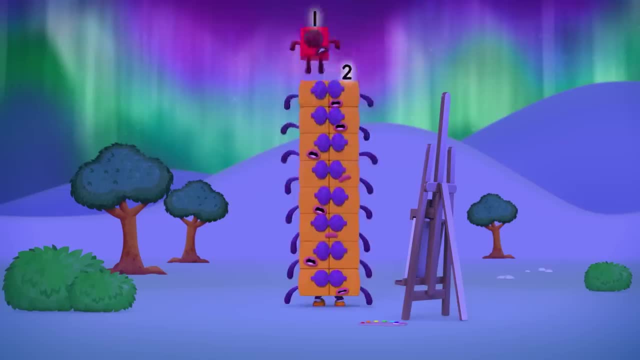 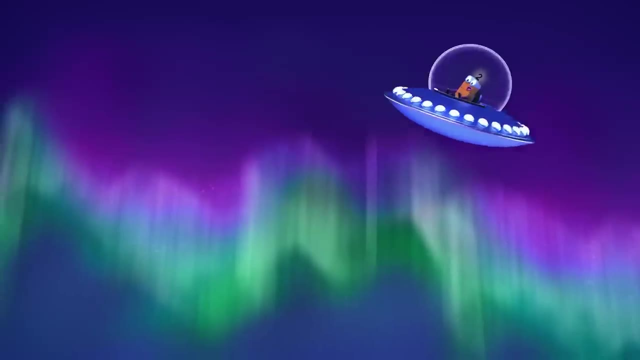 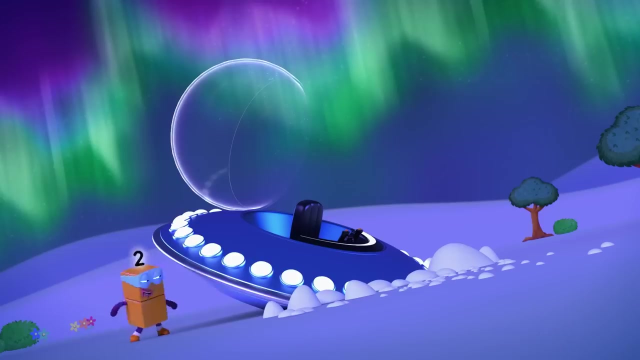 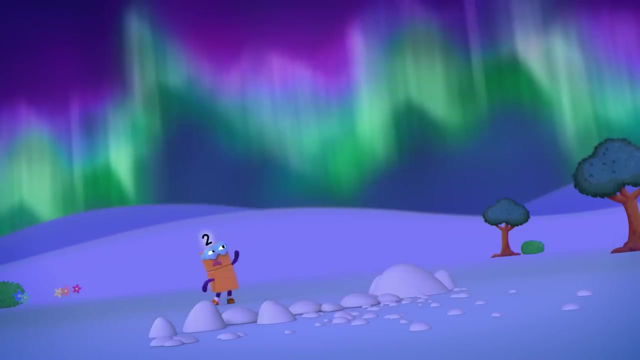 Remainder one. No Run Ten experience. I must paint it. Whoa, Whoa, Oh. Uh, where's that reset switch? Aha, Oh, You've got to hand it to me, Whee Hey. 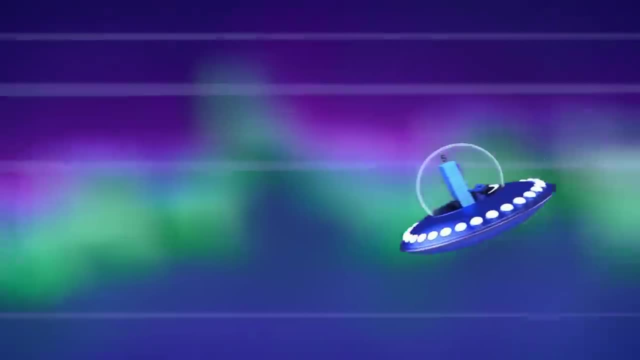 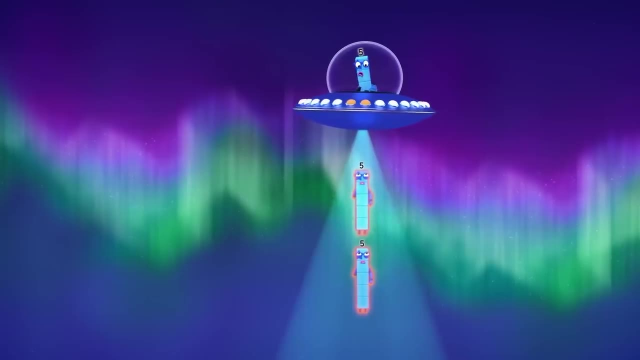 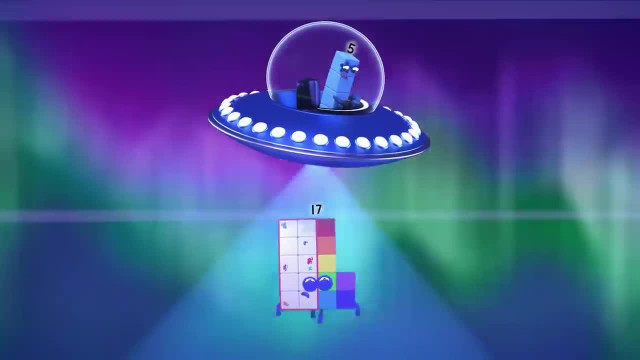 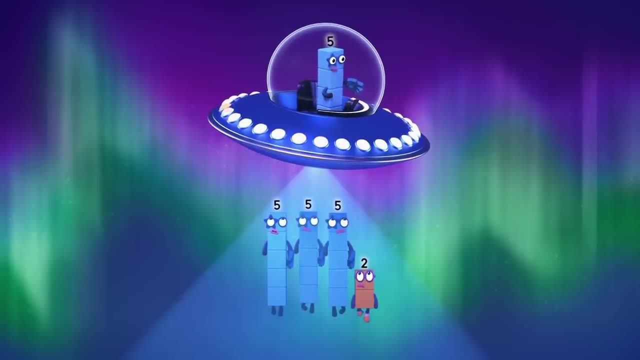 Huh, Huh, Sorry, Learn a driver. Remainder alert. Remainder alert. There are three fives in 17 and two left over. Remainder two: Whee, I think I've got the hang of it now. 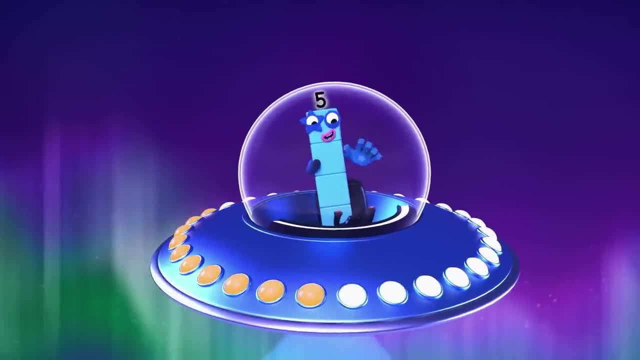 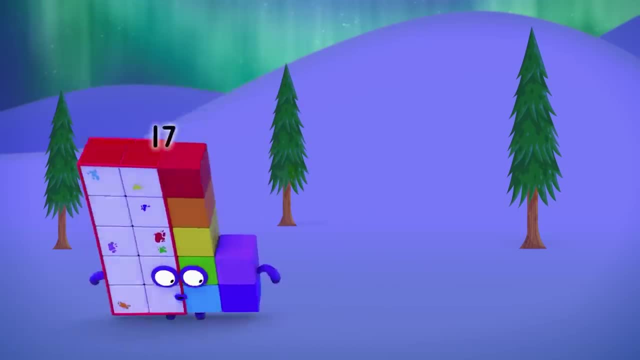 The twos factor beam divides you into twos and my factor beam divides you into fives, But only if there are no blocks left over. Whoa, Whoa, Whoa, Whoa. What, What can I say? There's just no dividing some people. 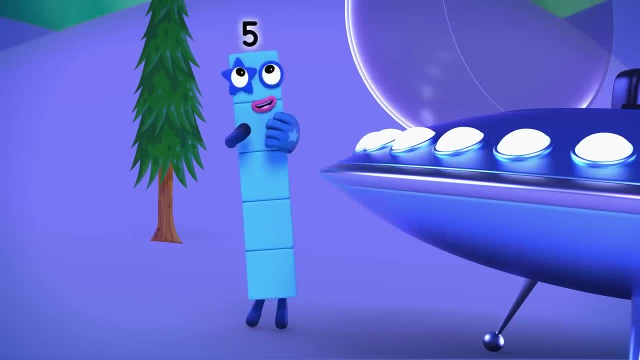 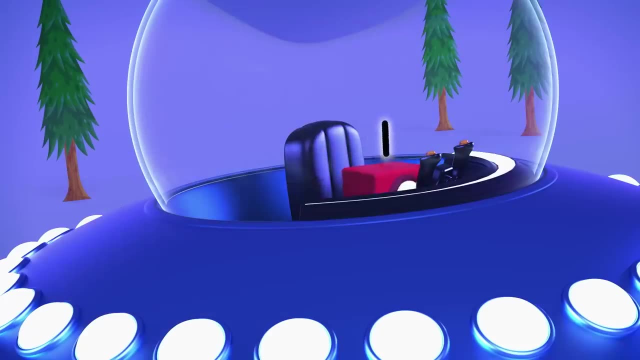 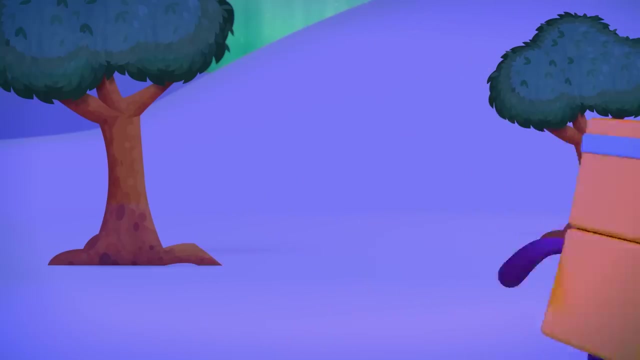 Ha-ha, I know how to stop the terrible twos And I know who can stop them. Mission accepted: Factor beam reset, Divide into ones. Uh-oh, Ah, Oh, Oh. How many ones in two? Two, of course. 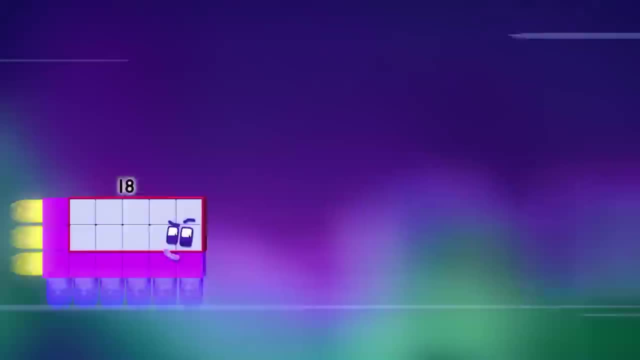 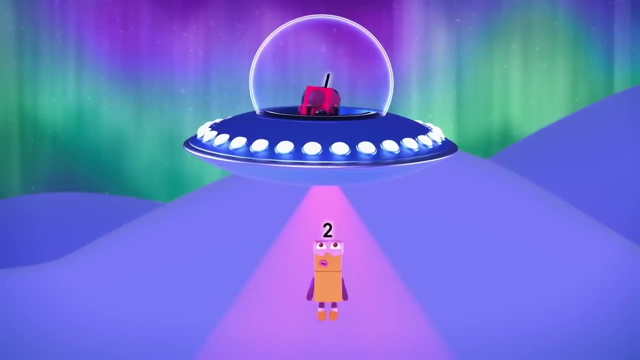 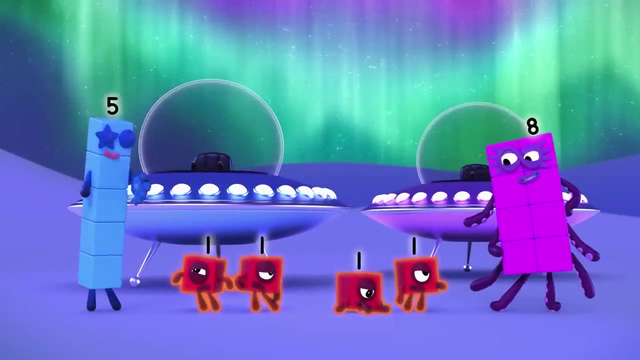 Ah, Double Bah, Whoa, Ha-ha-ha-ha-ha. Oh, Oh, Whoa, Never any remainders when you split into ones Bah, Well, well, Aren't you the naughty ones, Ha-ha-ha-ha. 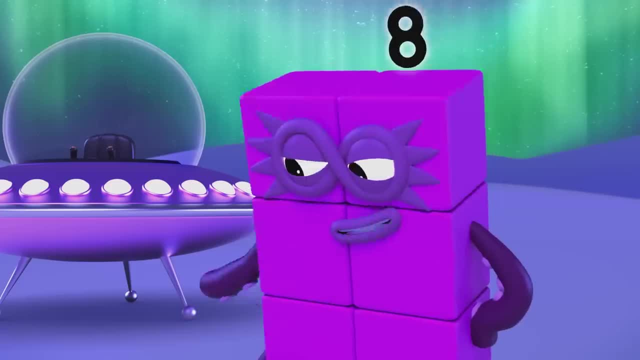 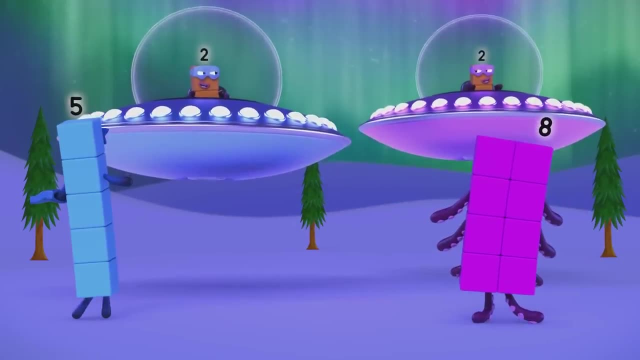 Don't worry, The factor beam wears off in time. Well, I don't think we'll be having any more trouble from. Wait, Where have they gone? Ha-ha-ha-ha-ha-ha-ha-ha, Watch the skies. 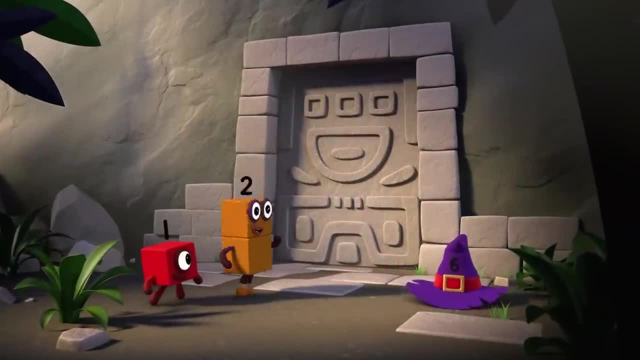 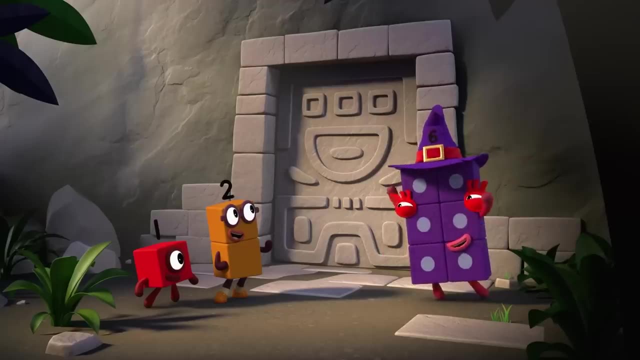 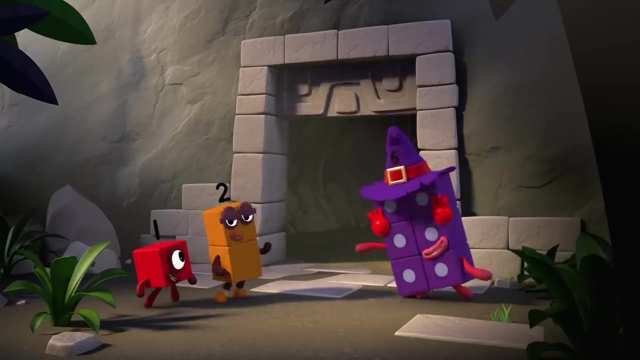 Whee, Whee, Ha-ha-ha-ha-ha-ha, Greetings all. Let's see who dares to step inside the lair of shares. Solve the puzzles, but beware: The treasure goes to those who share. 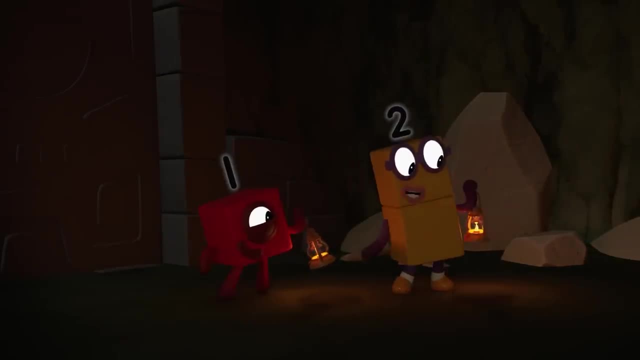 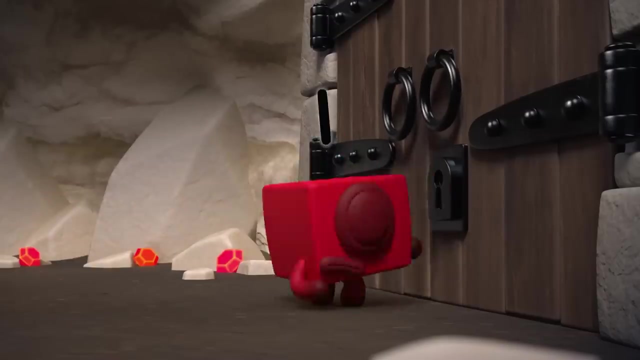 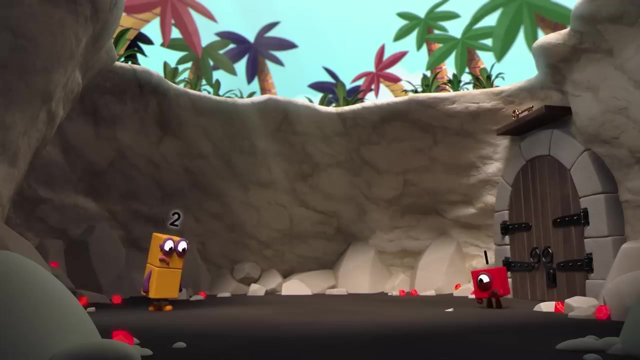 Ha-ha-ha-ha-ha-ha- One for you and one for me. Wow, Ooh, It's locked. Look, there's a key, But how do we reach it? I am the genie of the air. 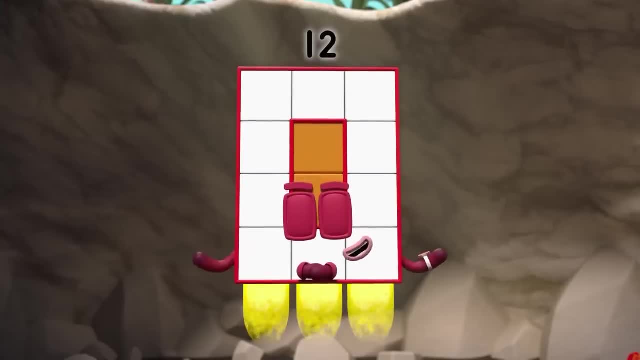 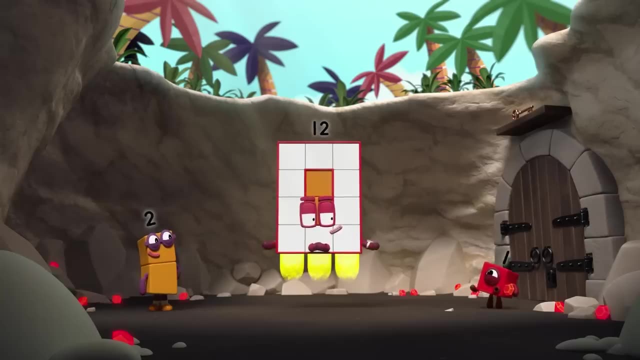 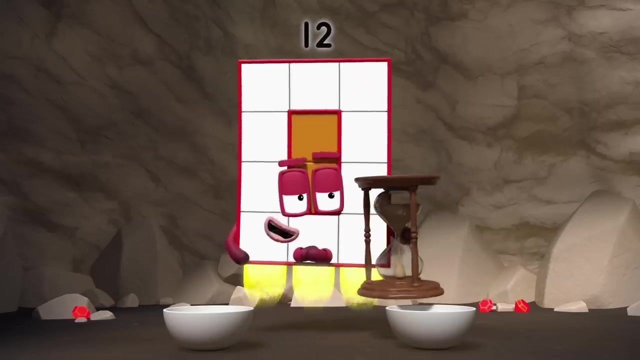 Ooh, To win the first key you must find all of my gems, Hee-hee. But to make things trickier, you must share the gems equally between these two bowls And hurry. When the sands of time run out, a bird will fly off with the key. 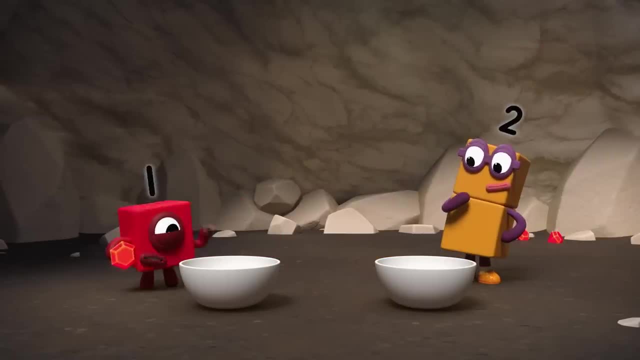 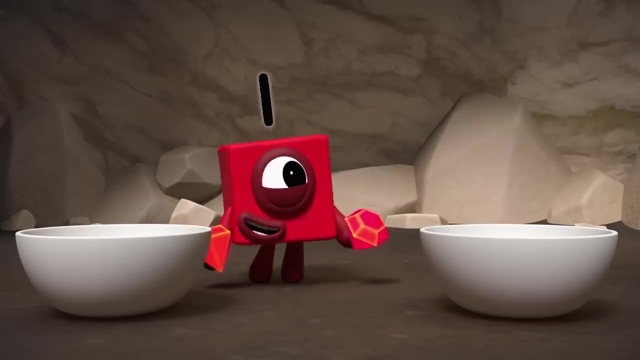 How can we put the same number in each bowl if we don't even know how many there are? Remember how we shared the lanterns: One for you, one for me. Yes, If we put one gem into each bowl in turn, they'll always have the same number. 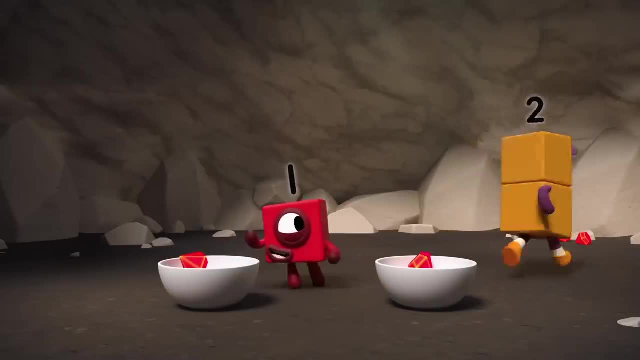 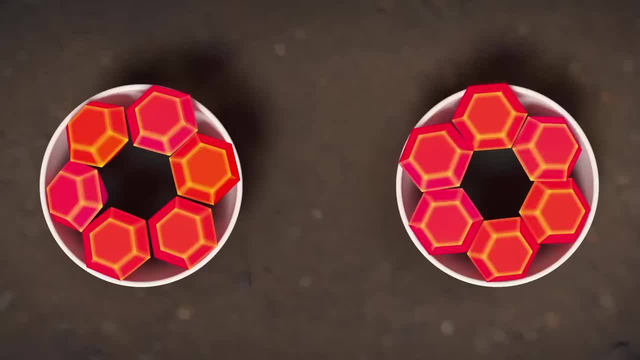 One for me. That's all of them. There are six gems in my bowl And six in mine. That's 12 gems altogether. That's right, 12 gems. Shag, be on your way. Shag be on your way. 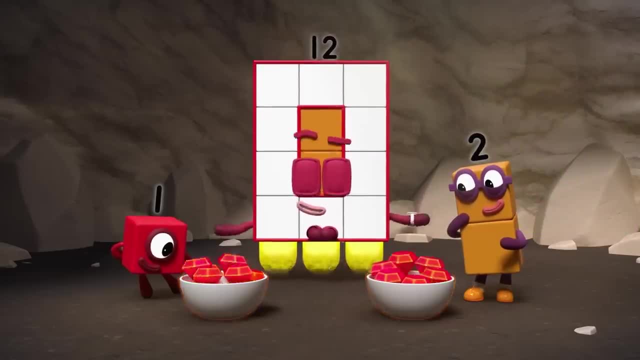 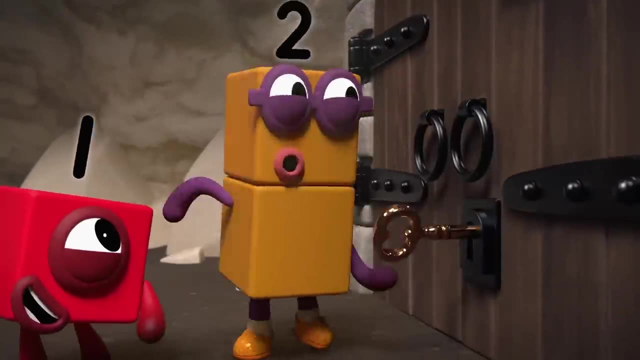 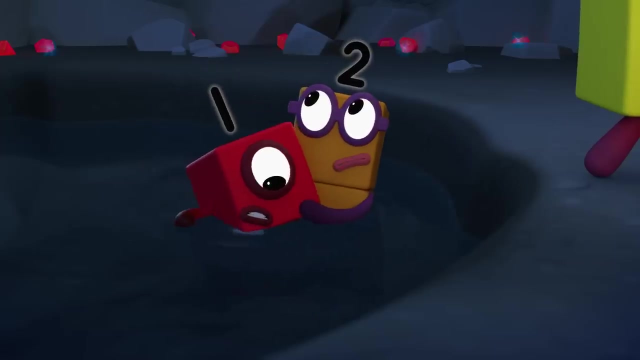 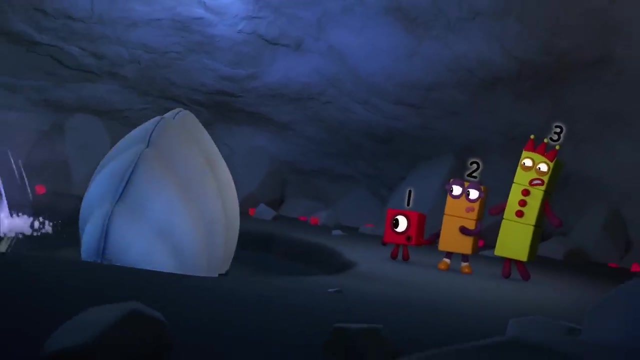 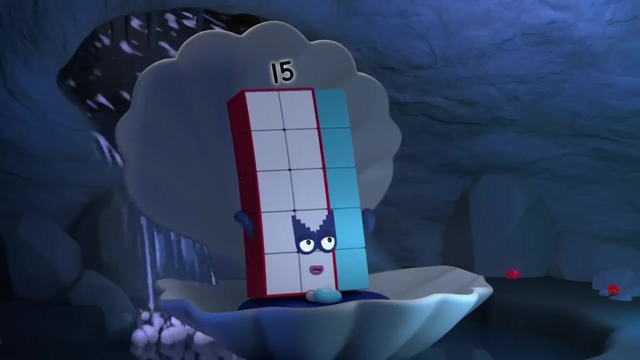 Shag, be on your way. One gem divided between two bowls is six in each bowl. Congratulations All right, There you are. I thought you'd never get here. I am the genie of water. Your next challenge: Share my 15 watery gems between these three shells. 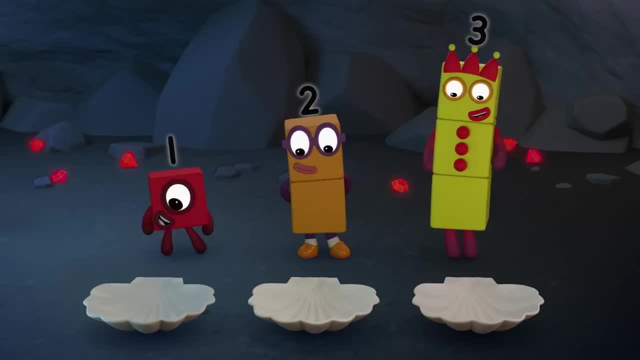 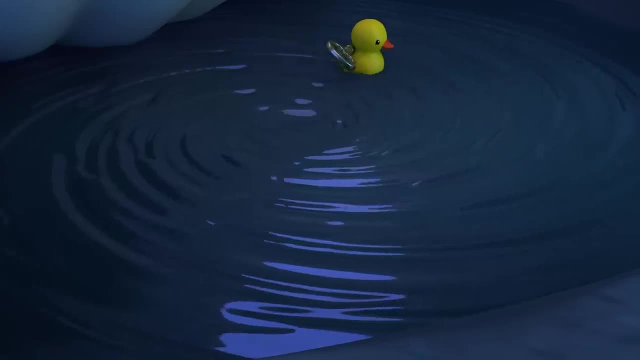 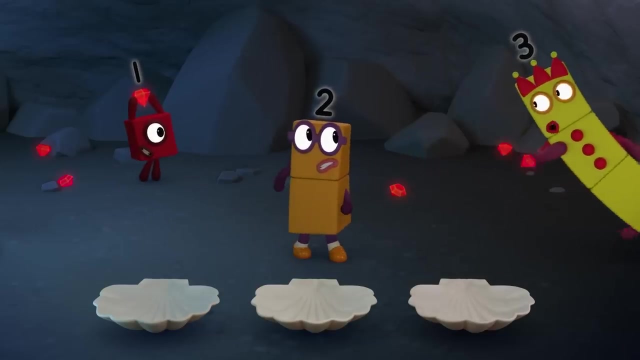 so each shell has the same number of gems. The next key: Share the gems before the waters run dry or the key will be sucked down the bottomless plughole. Quick. One gem at a time. No, no, no, that's too slow. 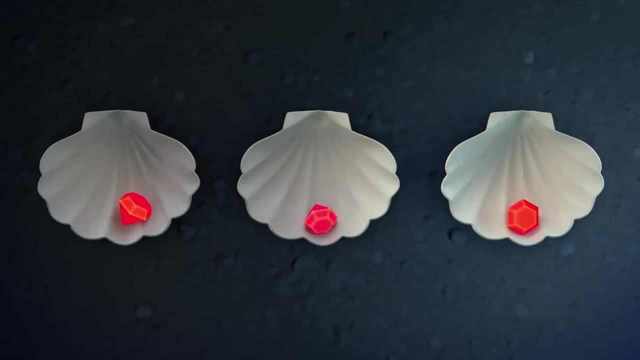 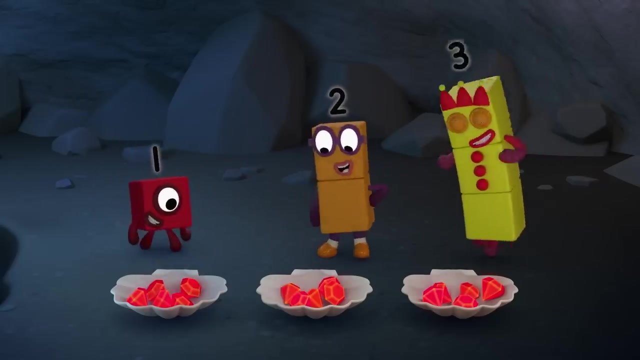 Let's get three at a time. Three shells, three gems, One gem in each shell. Good thinking, Three, Three shells, three gems, Two gems in each shell. Each time there's one more in each shell, Three more and three more, and that's all of them. 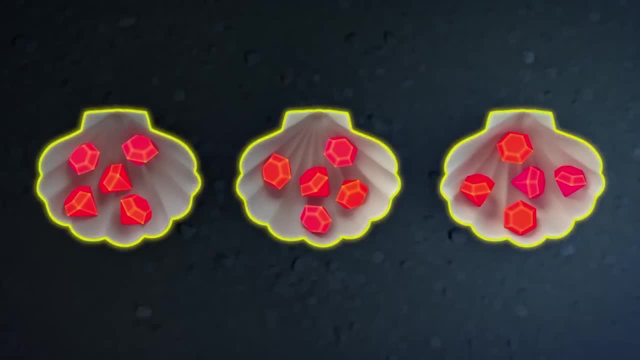 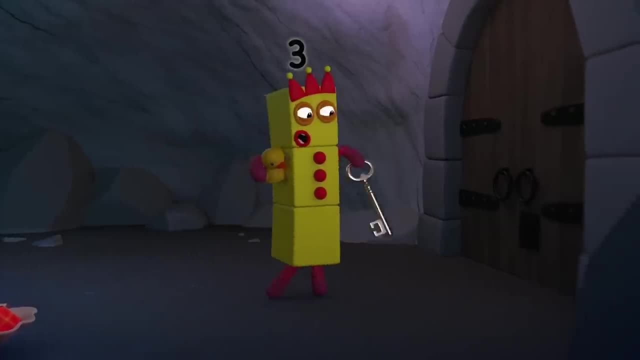 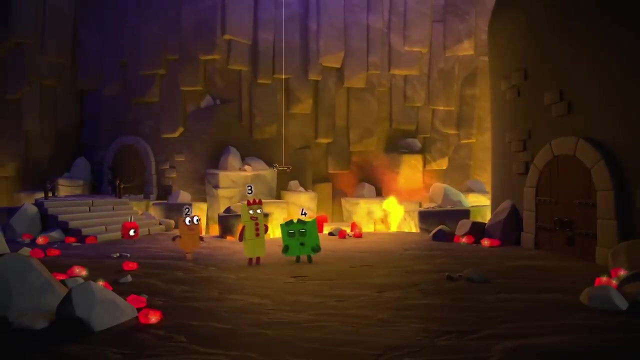 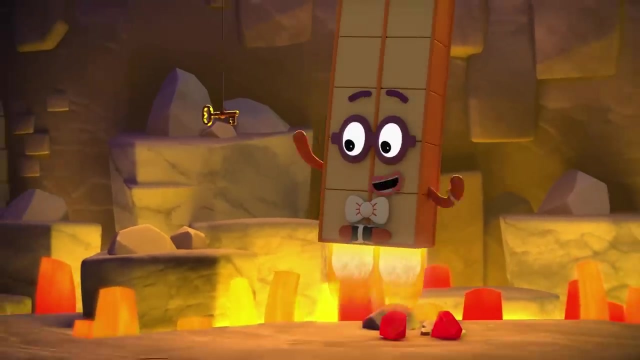 Oh, 15 gems shared between three shells is five gems in each shell. Good sharing team. Hello Nice and warm. here I am the genie of fire. To win the final key, you must share my 20 fiery gems into these four chests. 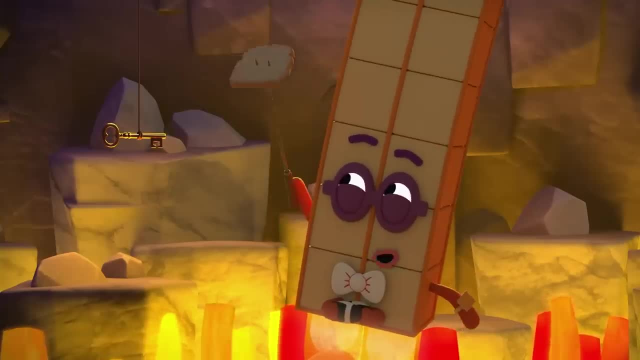 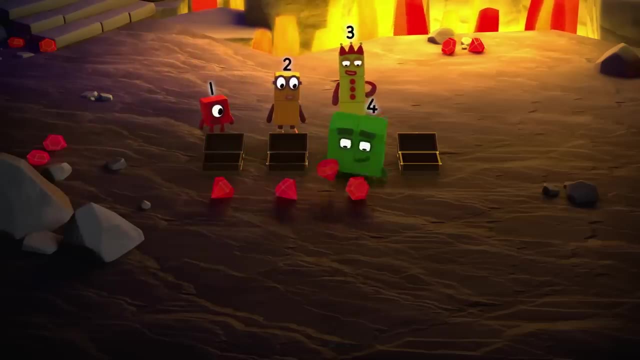 You have until my toast is ready, Go. We need to make sure we find all 20, so let's lay them on the ground as we go. Then we can check one for each chest. Now you put yours there. We need five rows of four to make 20.. 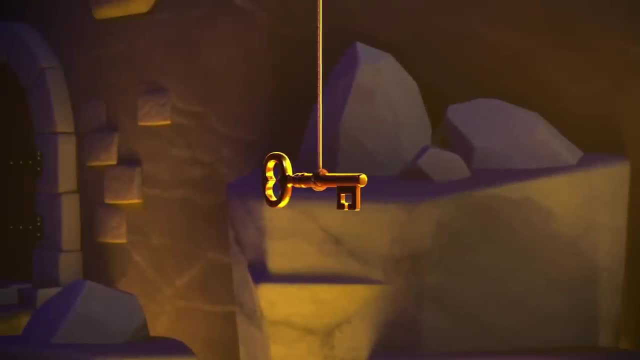 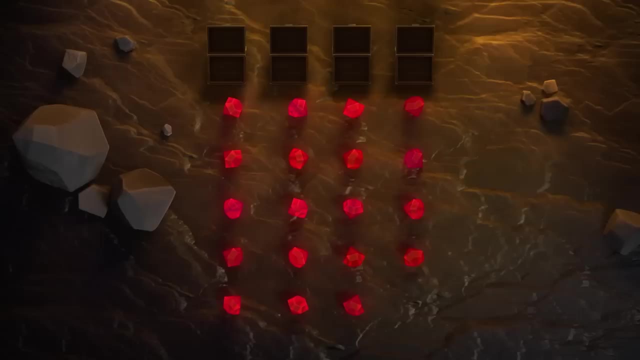 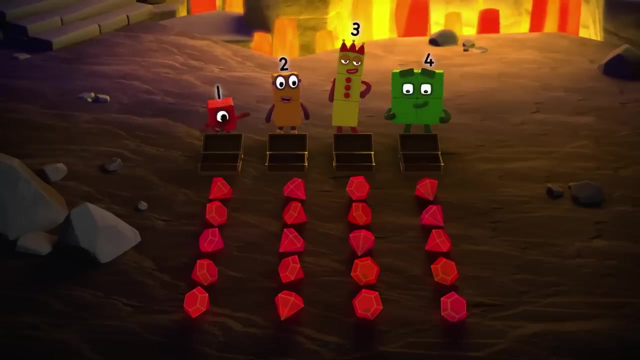 My toast is nearly done and the key is nearly toast. I can't see any more. Do we have them all? We can't have. Look, this line has one gem missing Here. Now all four lines are equal. That's right. 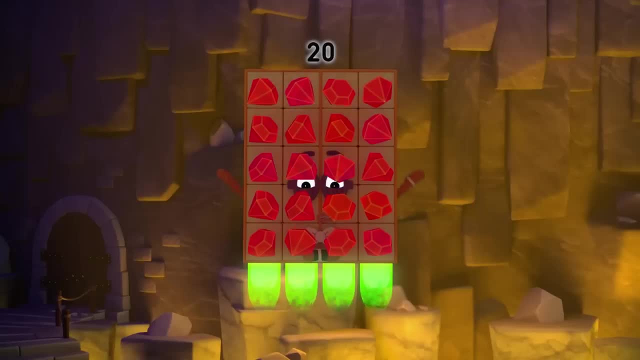 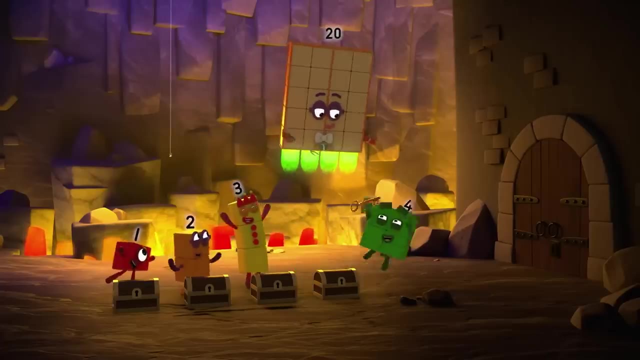 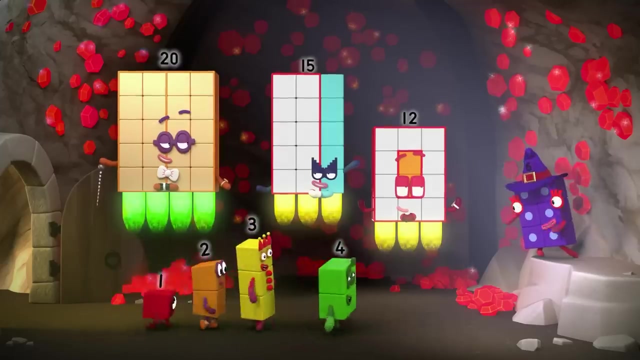 20 gems shared equally between four chests is Four, lots of five. You've won the game. Ooh, Gems of water, fire and air: Enough for everyone to share Yay.